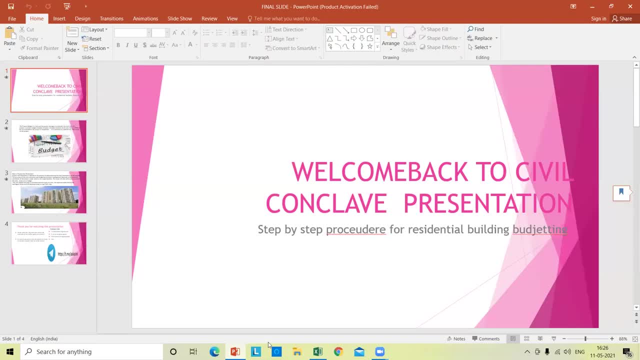 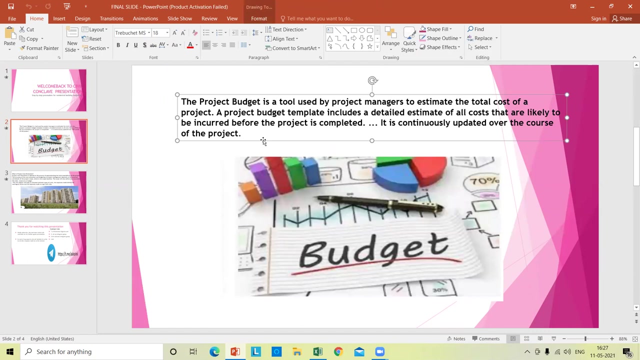 okay, now i have to. dear friends, welcome back to civil conclave presentations. today we are going to discuss about step-by-step procedure for residential project budgeting. the project budget is a tool used by a project manager to estimate the total cost of the project. a project budget template includes detailed estimate of all costs that are likely to be. 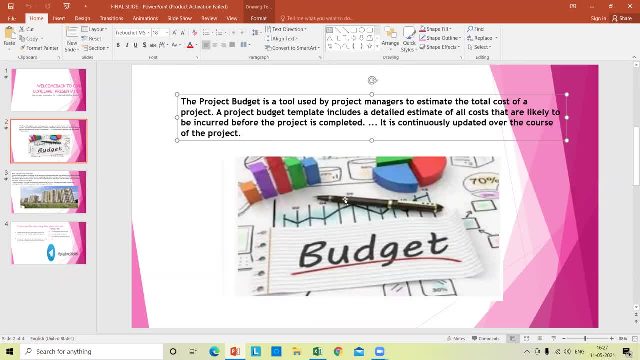 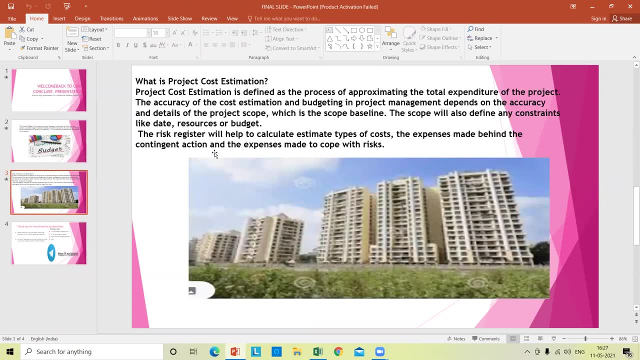 incurred before the project is completed. it is continuously updated over the course of the project. what is the project cost estimation? project cost estimation is defined as a process of approximating the total expenditure of the project. the accuracy of the cost estimation and budgeting in a project management depend upon accuracy of the details of the project scope. 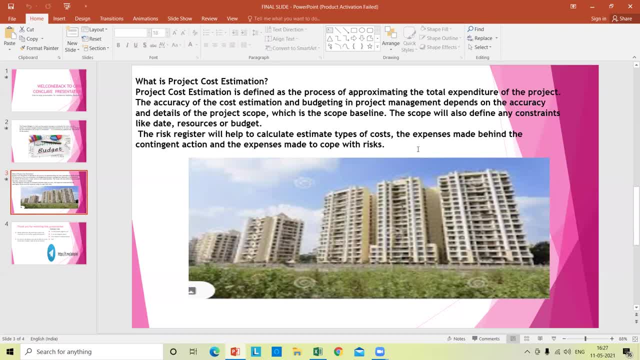 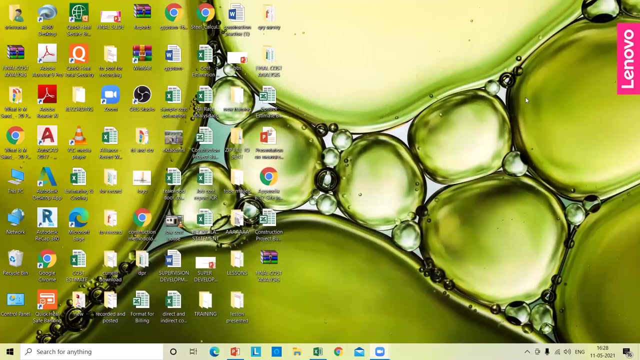 which is the scope baseline. the scope also will define any constraint, like date, resources or a project. the risk register will help to calculate the estimate of the type of the cost, the expenses made behind the contingent action and the expenses, along with the course that will be used to determine the total cost of the project. 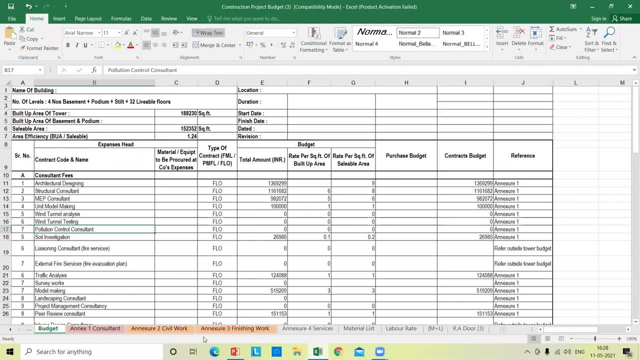 now let us go to the project budgeting. see, this is can be treated as only purely a template. it cannot be, because the rates bound to vary according to the today market prices and everything. so i give you a proper template: how to create the project budgeting. you can download this file. 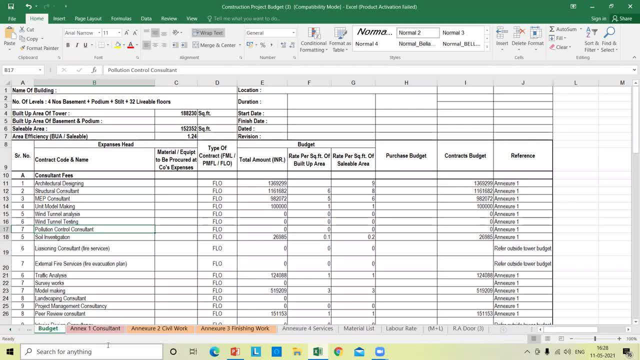 for which the link has been provided in the presentation. let us start with it say you have to mention the name of the building. where is the location? this is my project of four basements stilt under 32 usable floors. you have to identify the duration building built up area. this project is for me, so one lakh eighty. 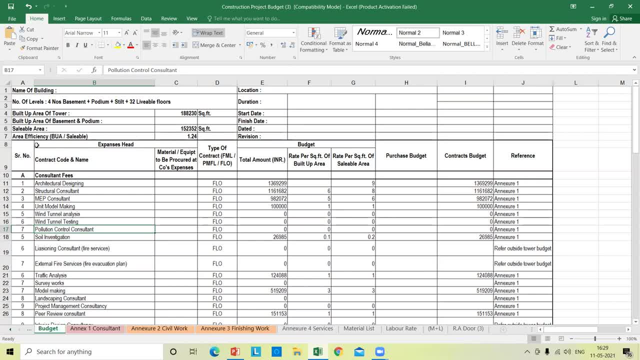 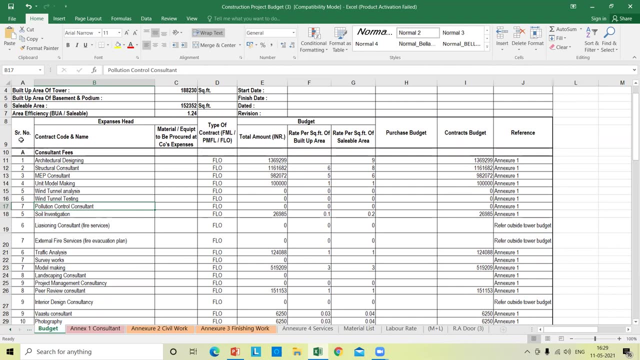 eight thousand three twenty. okay, sellable area- area efficiency. that means built-up area versus sellable. okay, now you have to come to create a such a system. where you have to create a such a system, you have to create a cost head. then the budgeting in the cost said: you'll be coming a contractor code. 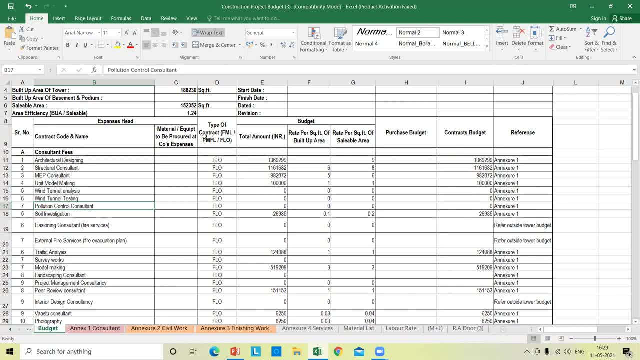 and name material equipments. type of a contract budget, you'll come to the total amount: rate per square feet of the built-up area, rate per square foot of the sellable area: purchase budget, contract budgets. this is the references. you have to identify it here. now let me go to the consultant fees. 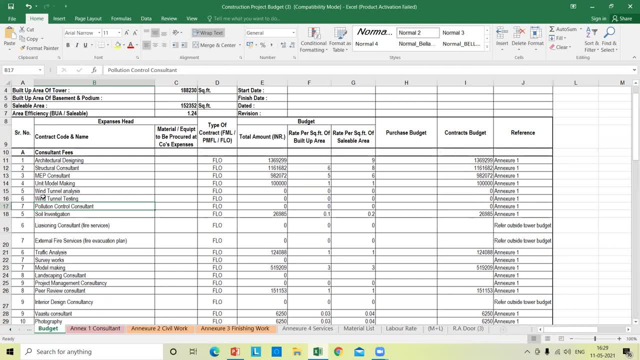 you have to go to the structural drawing. you have to go on filling it into all the columns. structural consultant: again you have to fill the columns mvp consultant: unit model making: what is the cost if there is a wind turbine? what will be the cost? podium control consultant: what will be? 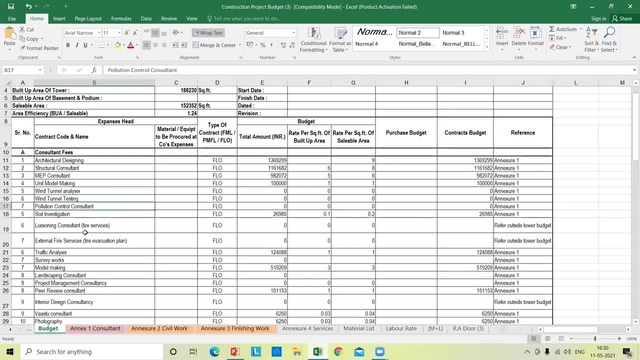 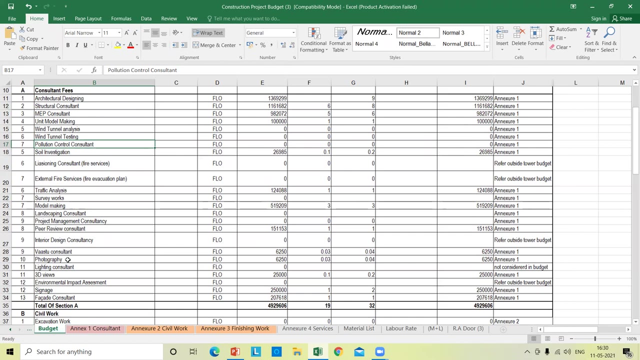 the cost? soil investigation. what is going to be the cause? licensing architect? what will be the cause? external fire services: what will be the cause? what will be the cause? survey walks? what will be the cause? model making, project management, consultancy, peer review, consultant, interior design consultant was to consultant photography. 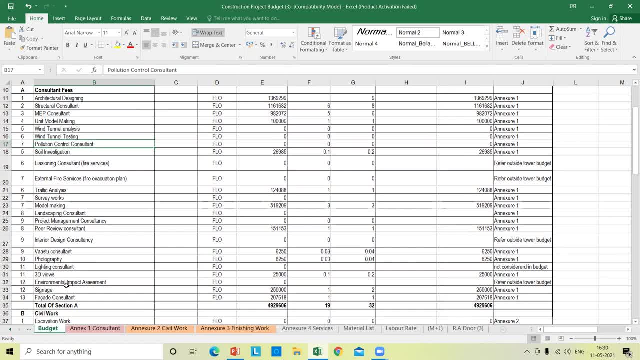 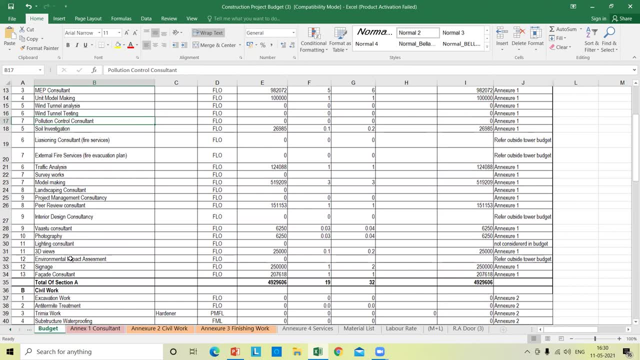 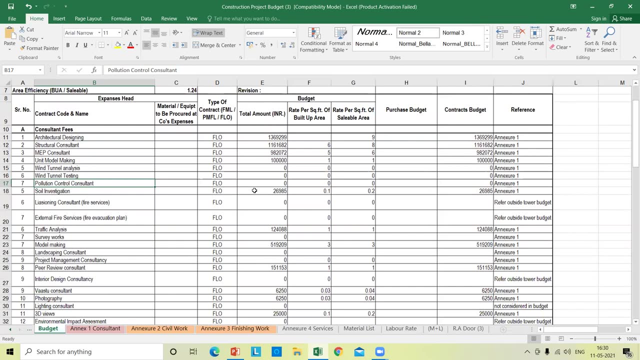 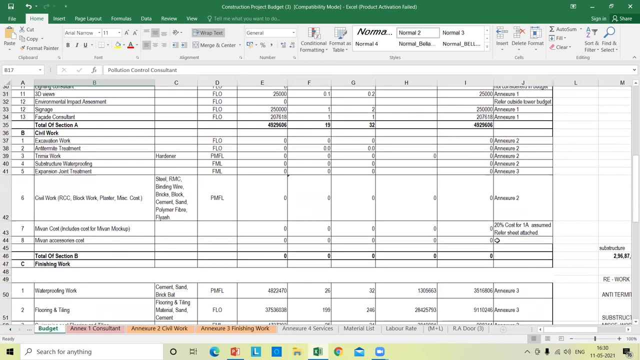 lighting consultant, 3d views, environmental and impact assessment, signage factor construction. this is a total work of all the consultant. this will be allocated for what will be the budgeting. you have to identify a total amount, budget rate per square foot built up area. you have to provide the annexures how you are deriving these figures. 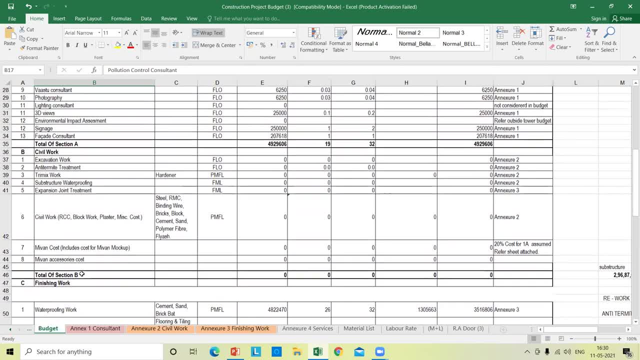 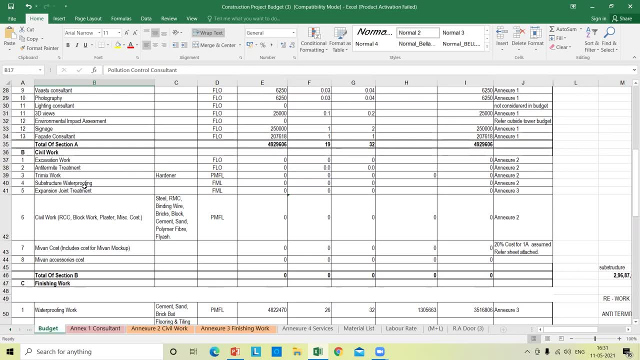 okay, this is. i'm calling it as section a. then comes to section b. this is civil works, where you will be considering excavation, anti-terrorite, tremendous uh substructure and waterproofing, expansion, joint treatment, civil works such as concreting, brickwork, plaster, etc. etc. if there is an aluminum formwork, you have to add aluminum. 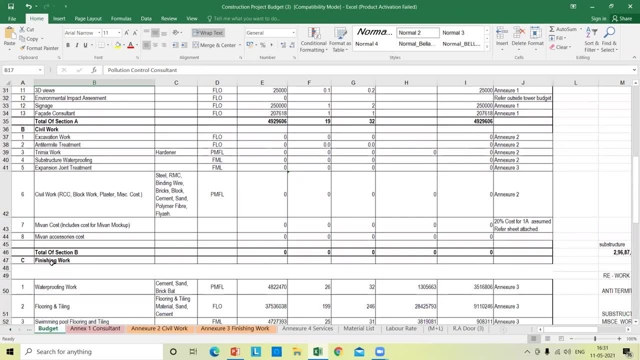 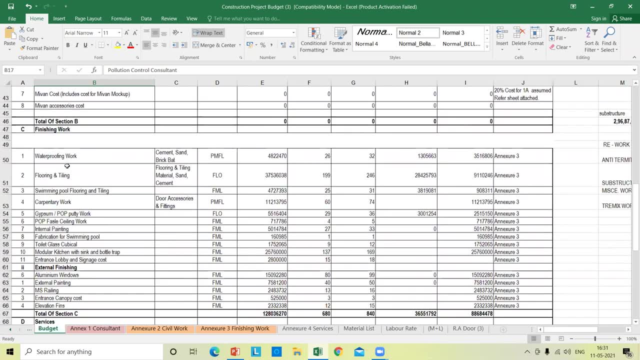 former aluminum accessories. this is cost. this total cost will be section b, which is known as a civil work. now come to finishing work. finishing work. what are the finishing works? waterproofing, flooring, tiling, swimming pool flooring, carpentry works, gypsum pop, false ceiling, internal painting, fabrications of swimming pool, toilet, glass control, modular kitchen, etc. then comes the 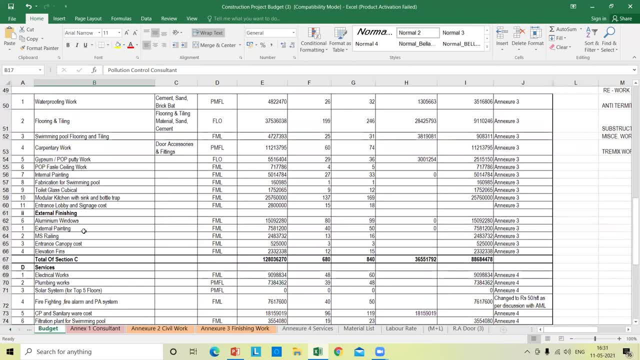 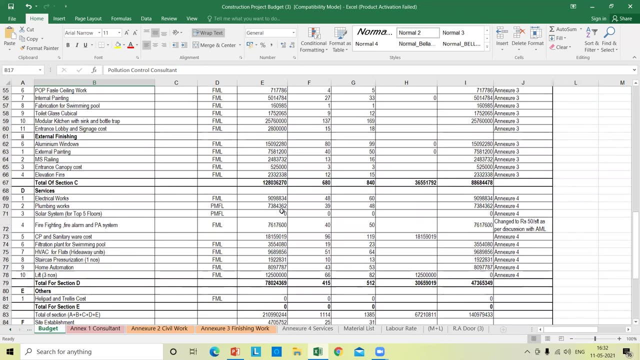 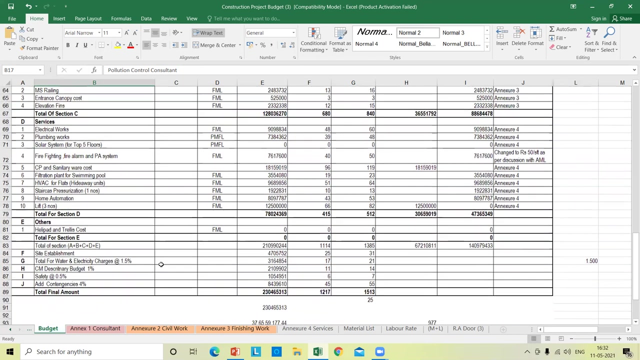 external finishing, aluminum fixture, external finishing, ms railing, entrance canopy, then elevation films. this will cost you the finishing item. then we come to services in services. what are the things covered? electrical, plumbing, solar system, firefighting, cp, sanitary, hydrate filtration plant, havc, staircase pressurization, home automation, lift, etc. this is called as services. now comes to others. 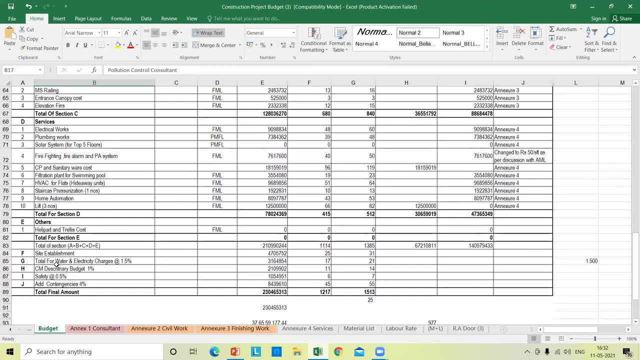 if there is a helipad or anything, you have to put it here. so total for will be: this will be of all the abcde, you'll come down to your figure. what will be your budgeting? then you have to add the cost right: establishment total for water and electricity. what will be the cost? uh, 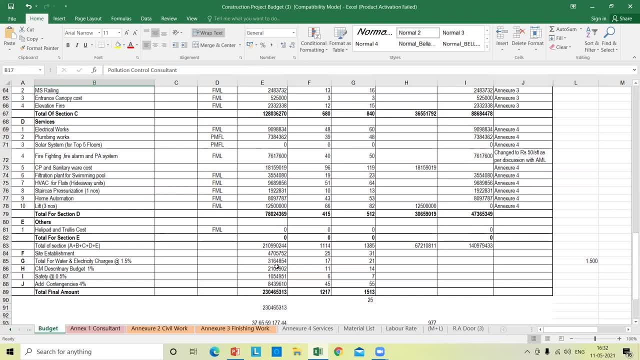 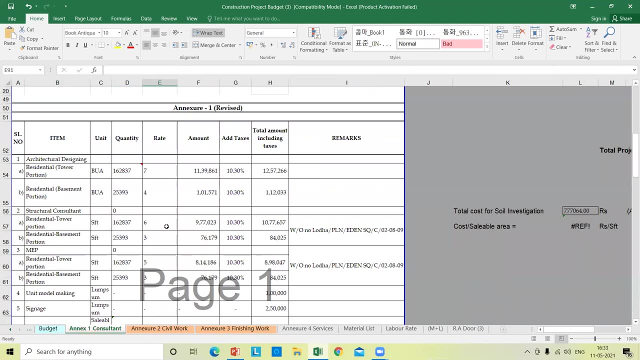 directory budget. what will be the cost? safety, what will be the percentage you're going to spend it? add contingencies, you add it, so the total final amount will comes to outdoor current. now we come to the consultant factors. consultant factors: how they are going to work out architectural designing. you have to mention unit, the quantity. 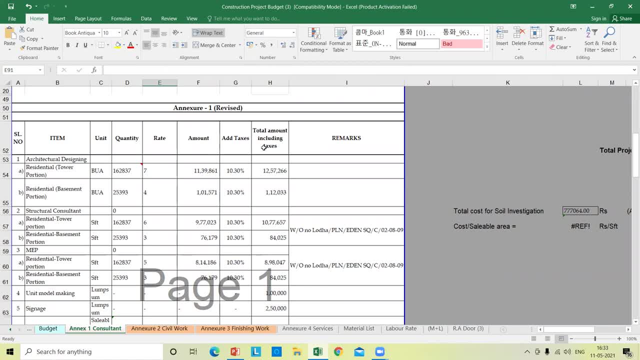 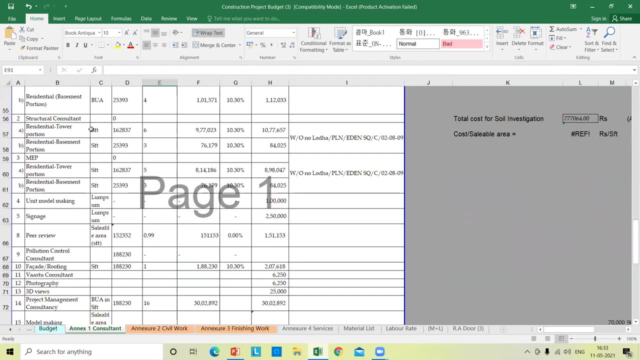 will be the rate amount, add taxes, then the total amount. okay, if there is no remarks, you can put it in the remarks. see, like this: residential tower. what will the built-up area, etc. etc. basement portion. what will be that? structural consultant for a residential tower? how much i paid residential 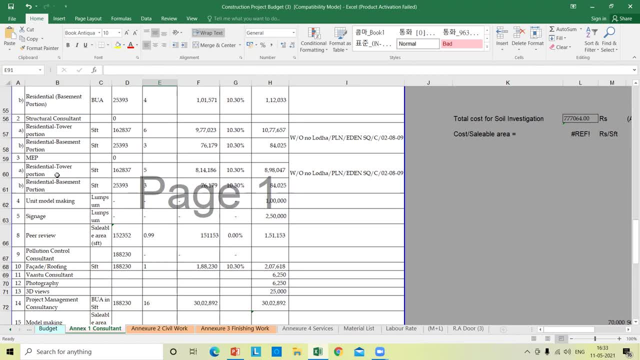 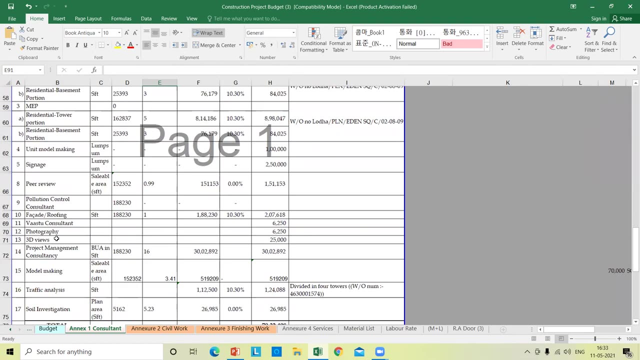 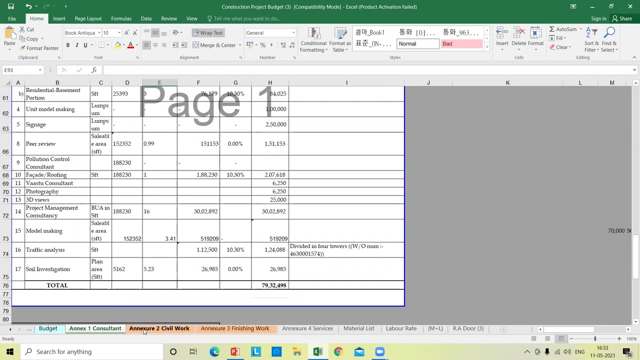 basement. how much i paid. again, mep. i split it into two parts. one is a residential tower portion, residential basement portion: model making, signage, peer review, pollution control, facading boss, consultant photographs, project management, consultants, and this total will make you the consultant expenditure. now we come to civil works. civil works, what? how do you are? 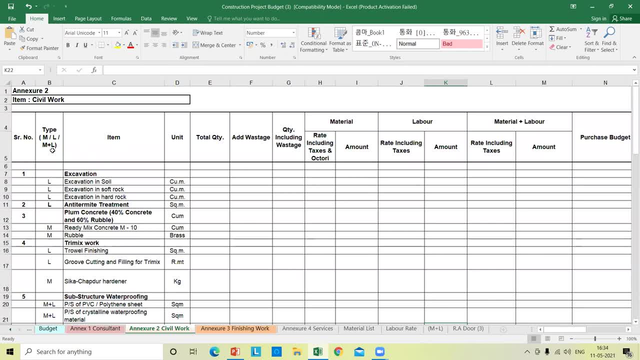 going to make it out. you have to mention that is a material plus labor or only a labor. the item description unit: the total quantity add wastages. quantity including wastages. now you have to segregate this into material and labor rate, including taxes and work. trial amount: labor: again the rate. 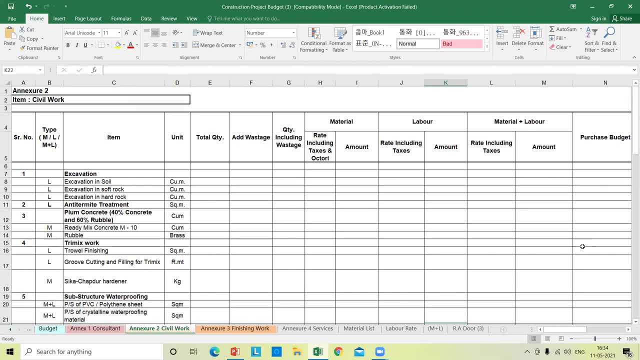 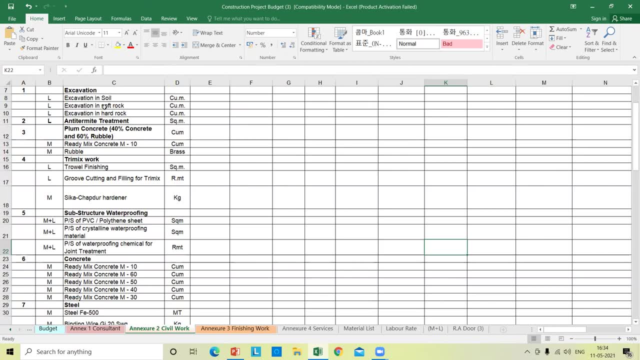 material plus labor, this. so what is the purchase budgeting? you have to provide it like this in civil items. i will separate it like this: only labor: excavation in soil, excavation in rock and everything: anti-thermal treatment. then come to see people's building tonight. i will let you flash tricks again. i will also provide anywhere. 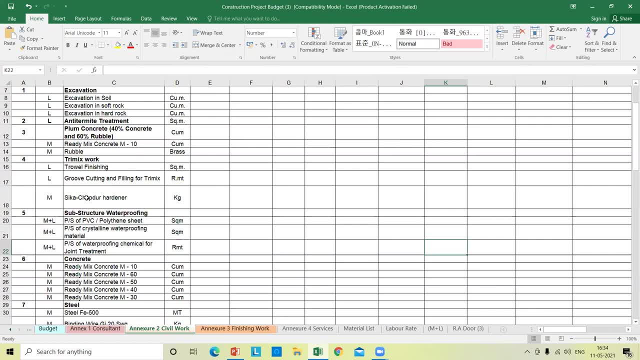 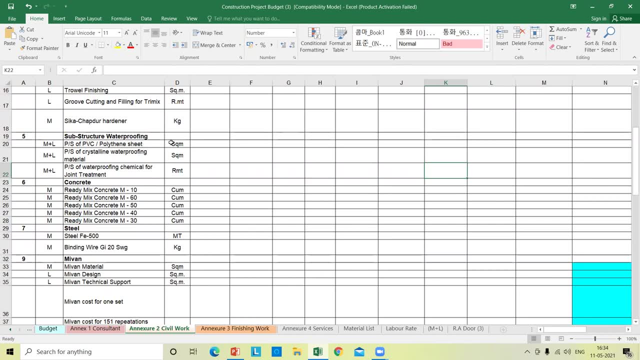 that your project actually has four. actually, this is very concrete material for the project. so the disgraving theory is that you put what the real reason for a concrete, the starting material in your building, which will be aisis, my thì, the building wise, not just for the same day. 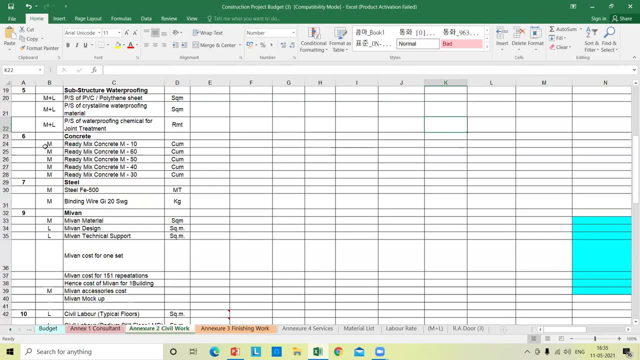 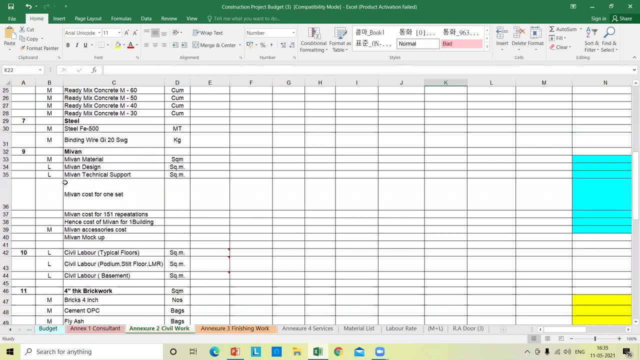 right, like, like, like. each building will be a six bedroom house, as this open ground. the clicking is mobile, is typeık spherical, but material. It's again a material contract: Binding wire. this is a contract. If we are using aluminum formwork for this budget, I use the aluminum formwork. 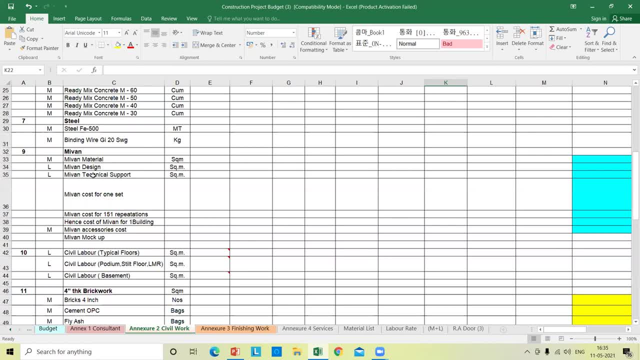 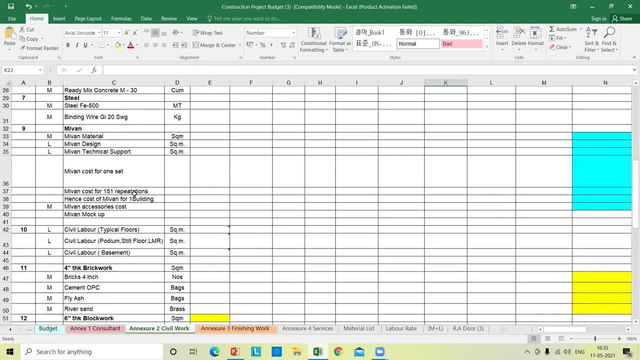 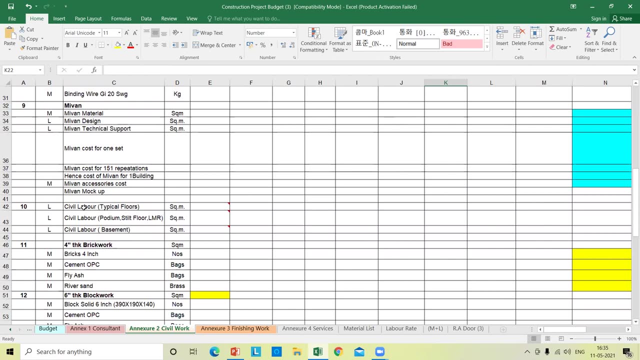 Here. aluminum formwork, what will be the cost? Aluminum design is a labor contract. My one technical support will be labor I consider as a 151 remediation. Then civil laborers for installing the shuttering labor first floor, what will be the square meter, etc. 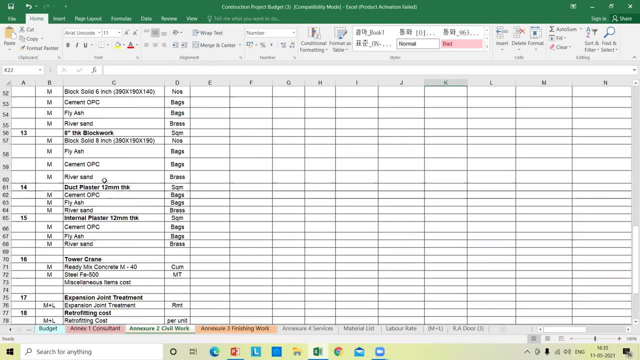 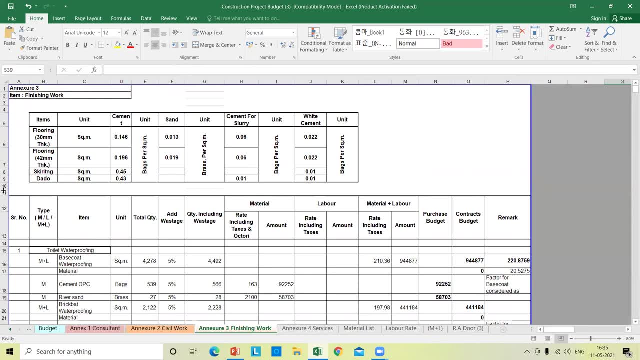 Like that. you have to go on brickwork and all these things. You have to segregate it out, material and labors accordingly. Then comes the finishing work. In the finishing work you have to segregate it out, All this identification. you have to give it what will be the coefficient of the materials? 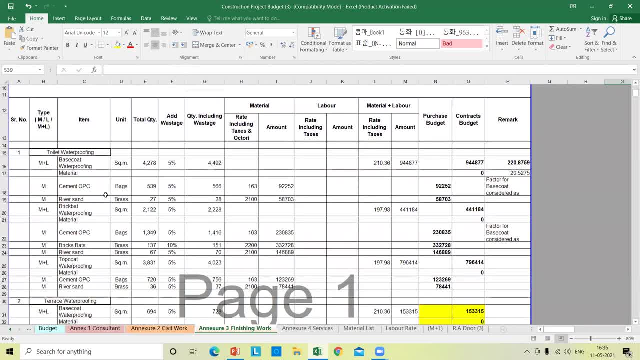 Like a cement. Now we come to waterproofing. Base code: It is the material plus labor. What will be the unit? The total quantity Add wastages, Quality, including wastages? What will be the material cost? What will be the labor cost? 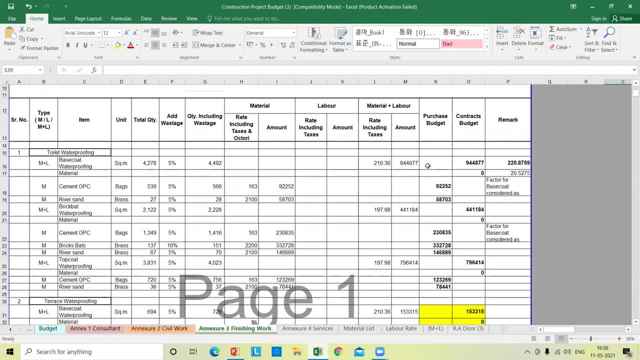 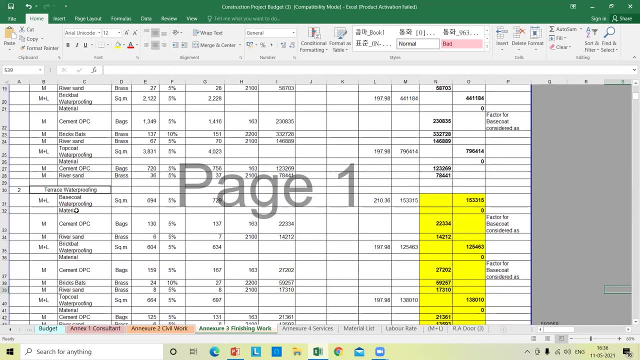 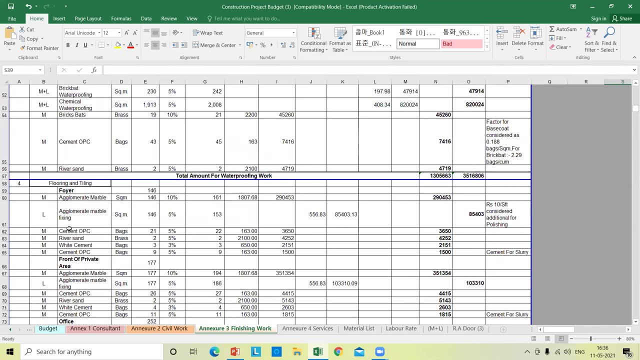 What will be the material plus labor? What is the project budget? What will be given to the contract? What are the remarks? you have to go on putting it out. It is like that: Terrace waterproofing- You have to go overhead waterproofing, swimming pool waterproofing, flooring and tiling. 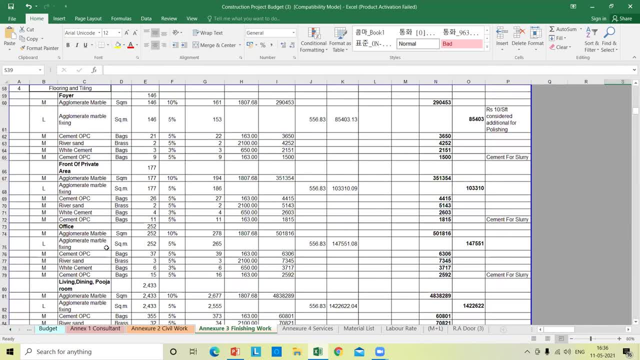 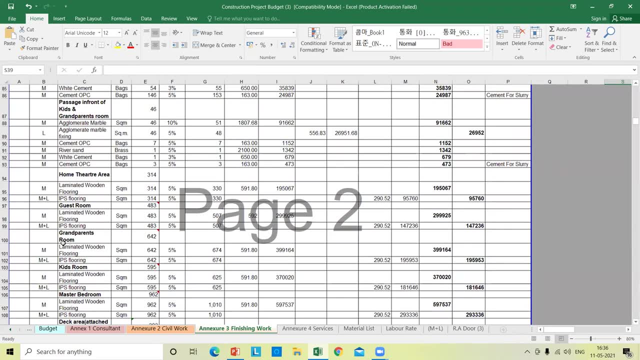 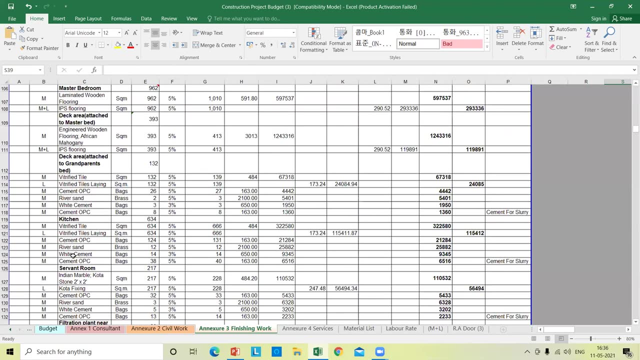 Again, the same methodology has to be adopted for all these items, Okay. Okay, Now, if there is anything else, like every room, you have to segregate it out. Every room, you have to mention it. What is the material? and etc. etc, etc. 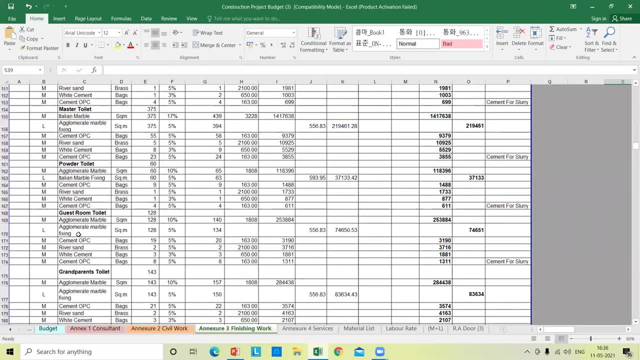 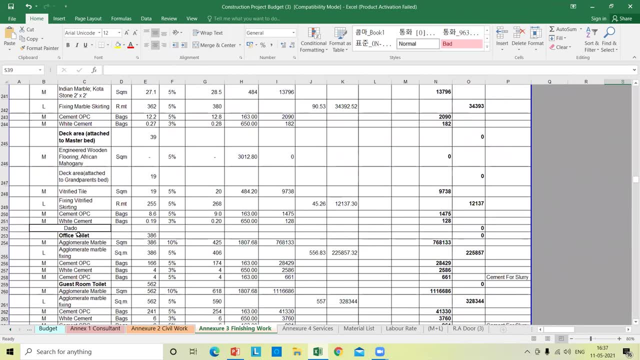 See, this is the entire brief I have given in this. This is the entire sheet which can be used. you can add, delete, hide anything. whatever you want to do, you can do it accordingly. you can create your project cost. 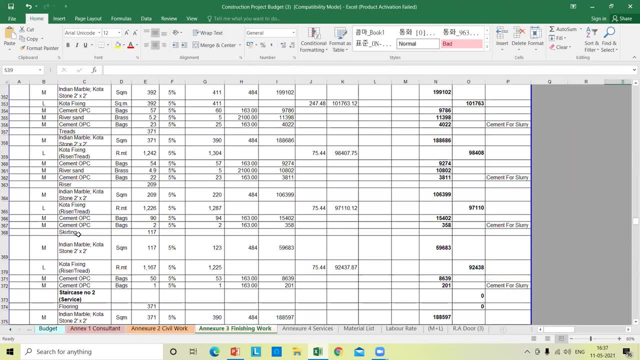 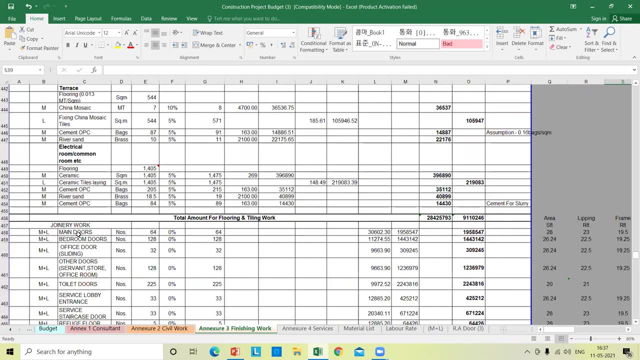 Okay, this is what we call as civil items, which is I segregated more than 500 items which will be helpful to you in creating your own items. Okay, then you come to total flooring and cost. Then you come for a project cost. 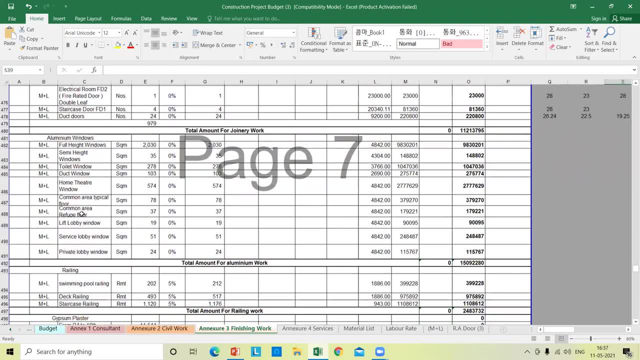 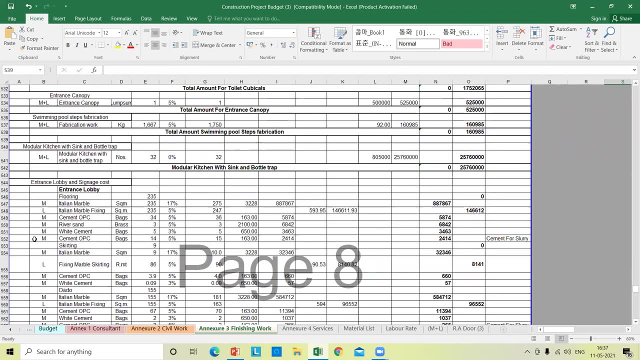 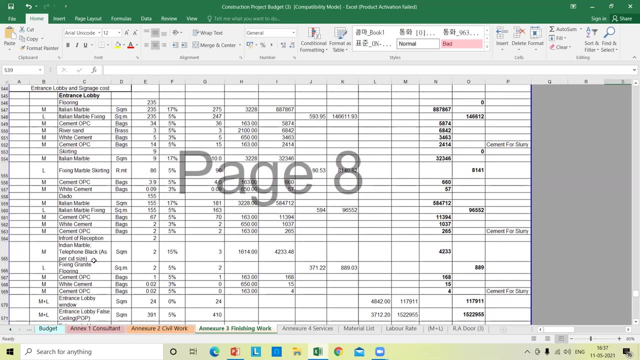 Then you come for a joinery box Like this. you have to create a joinery box, aluminum windows, etc. etc. You have to go on creating it. Then entrance lobby comes down. In entrance lobby, whether you are using Italian marble or any other marble, you have to go on putting it out. 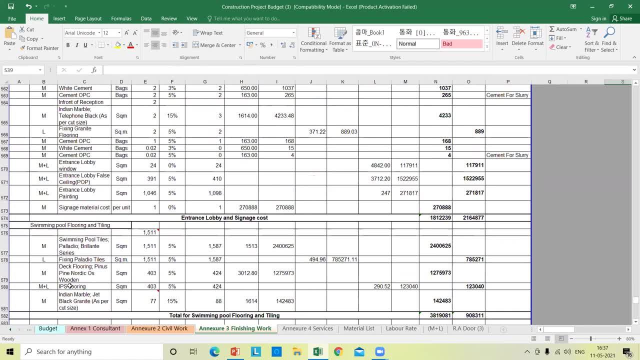 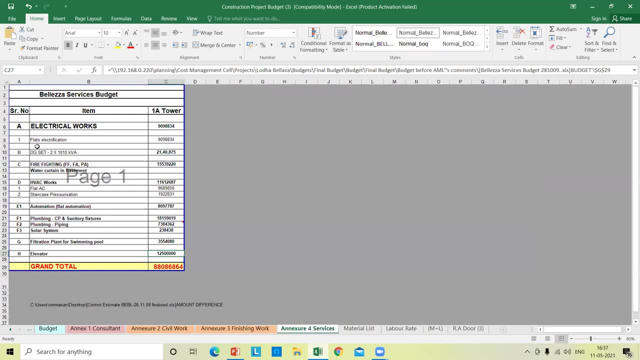 This is additional. Then signage board: Signage board. what will be the things? swimming pool, etc. etc. Now comes to services. In the services, electrical works, You have flats. what will be the cost? DG- what will be the cost? 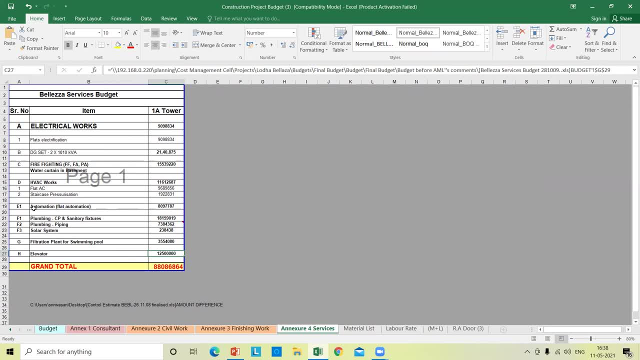 Firefighting- what will be the cost? HAVC: what will be the cost? Automation: what will be the cost? Plumbing and sanitary items: what will be the cost? Like that, you have to go on, add it. 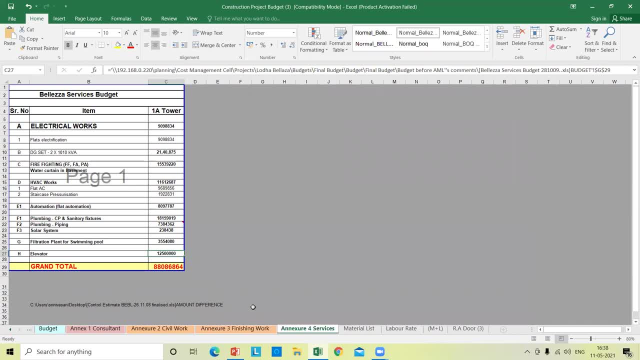 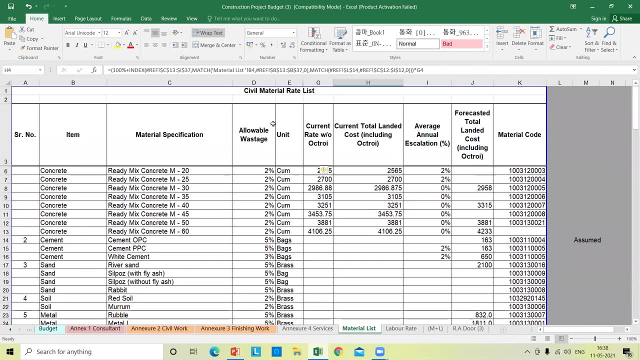 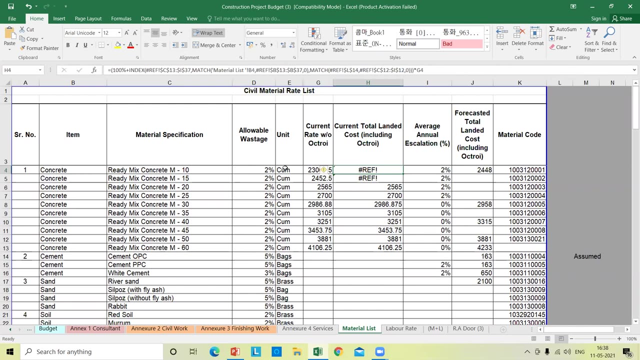 Then you come to a final cost of the services. Then it comes to material rate. Now you have to calculate for a material rate, Say concreting, what will be the materials Specification, what will be the wastages, the total unit- this is the current rate according to my project cost, then landed cost, what will be there? then add for an annual escalation. 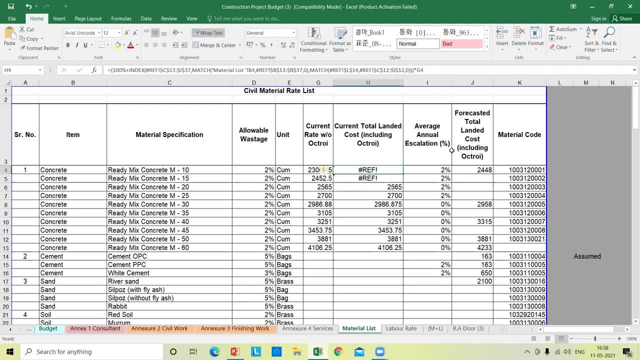 See here. this is the escalation is a tricky part Here. if your project is going to be finished within a short period, you don't add for an escalation. If the project is for a longer duration, you have to add on an escalation. 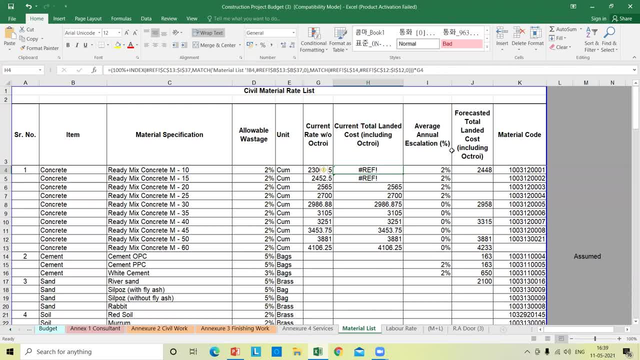 Suppose today the concreting rate is thousand rupees. After one year it might be 1100 rupees. So you have to add 10% escalation. for a second year Like that, you have to go on costing it which we call as a forecasted total cost. 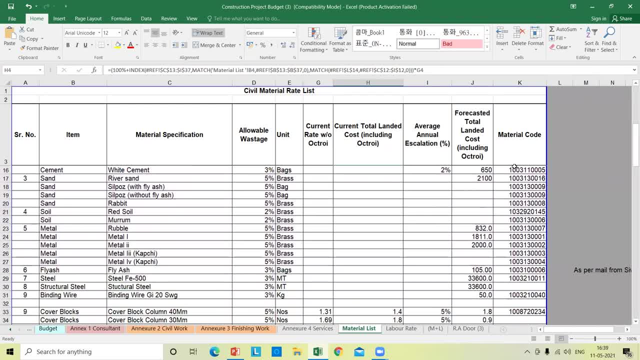 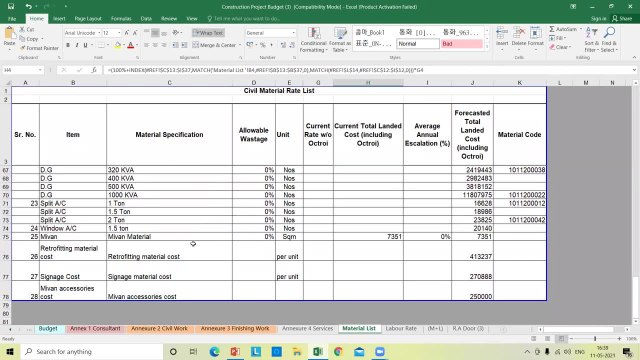 For your accounting purposes, you have to create a different code accordingly. For my projects I work on ERP, So I put it. on all these things: See, here you had all the items have been covered. Then we add a material cost, like this: 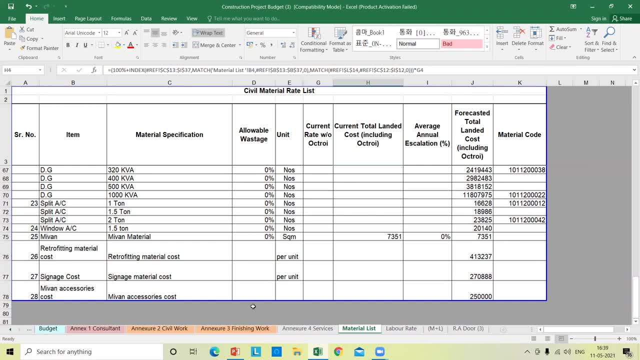 You add a labor cost also. You have to go on like this. You have to do it on. Where do I move this? I don't know if I can move this. It's green. 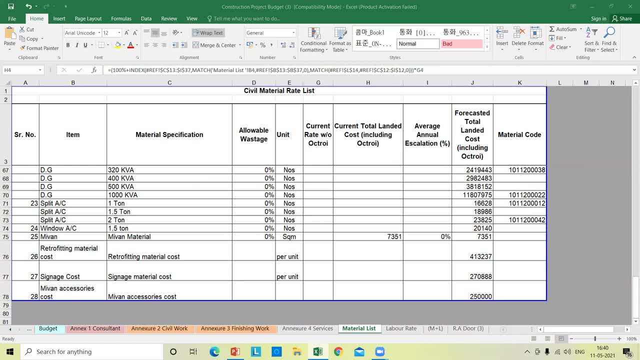 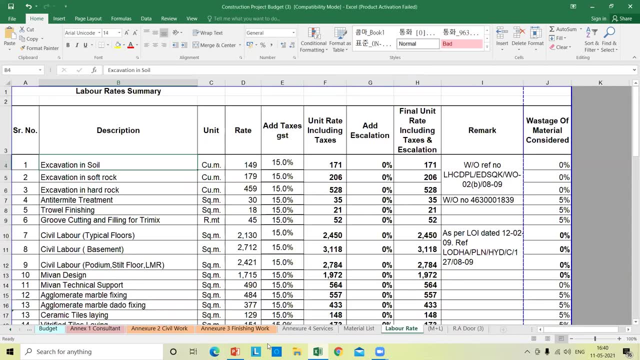 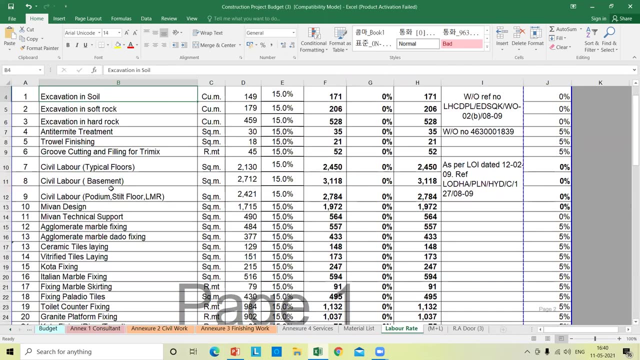 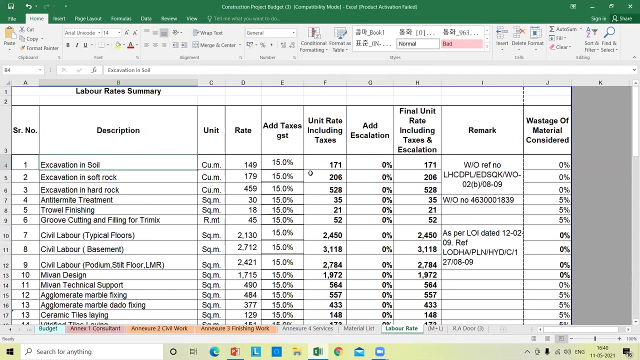 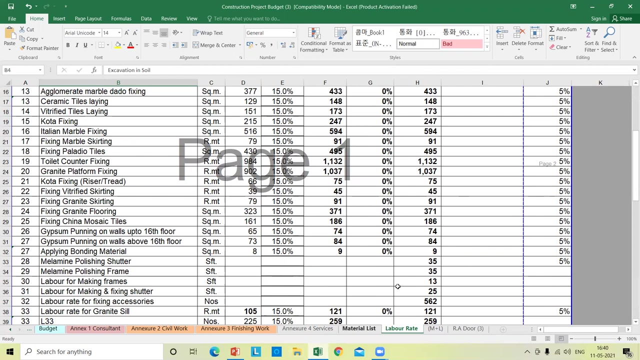 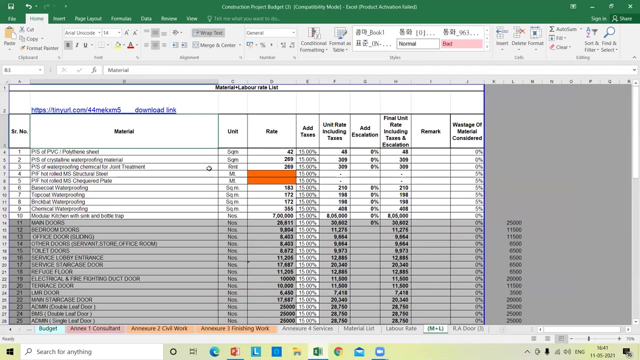 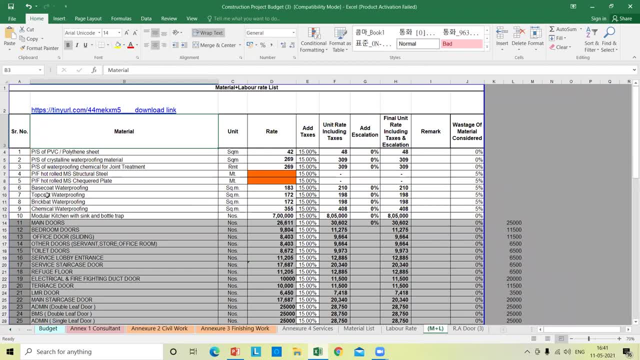 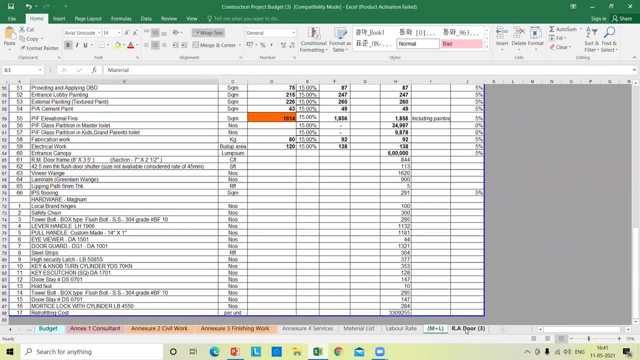 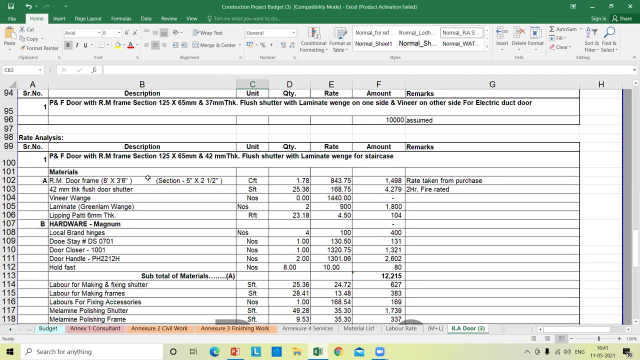 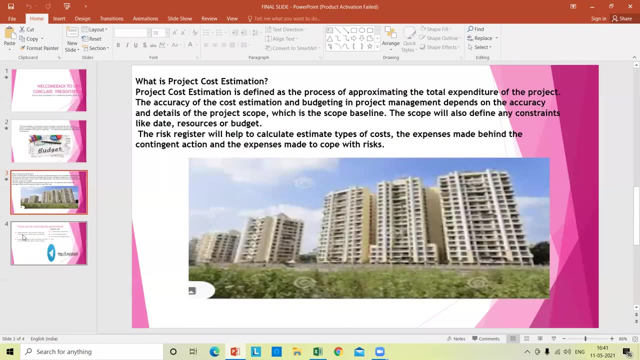 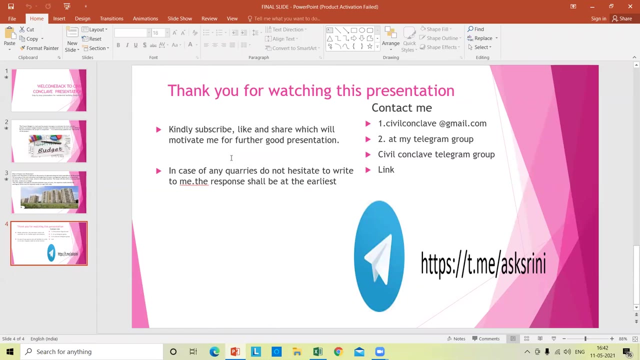